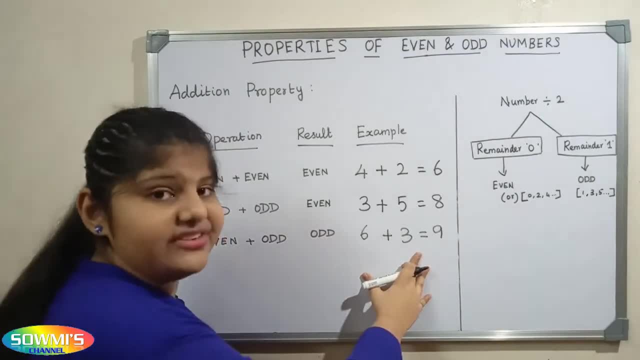 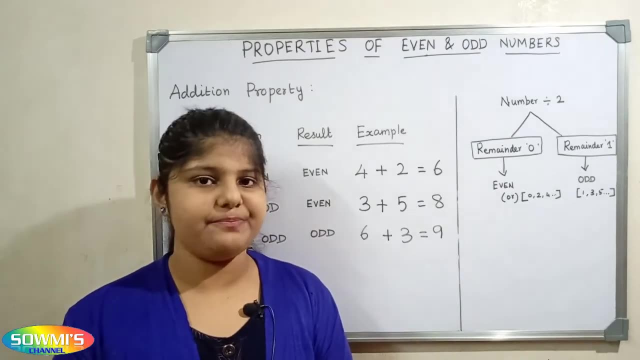 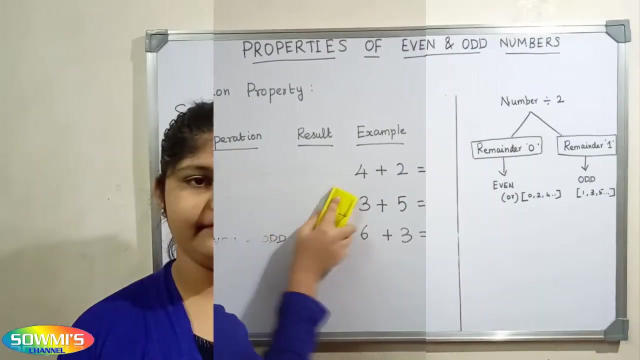 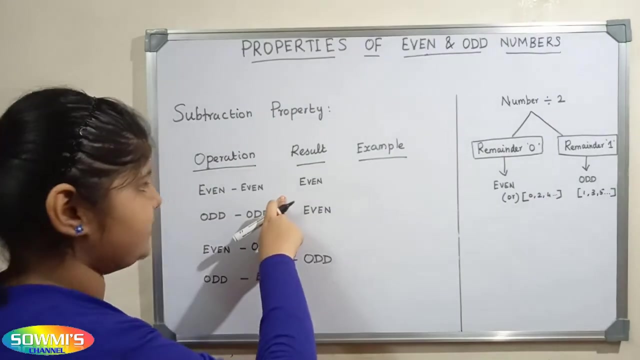 When we add 6 and 3, we will get the result as 9.. Here, 9 is the odd number. Next we will see subtraction property. Subtraction property: When we subtract two even numbers, we will get the result as an even number. 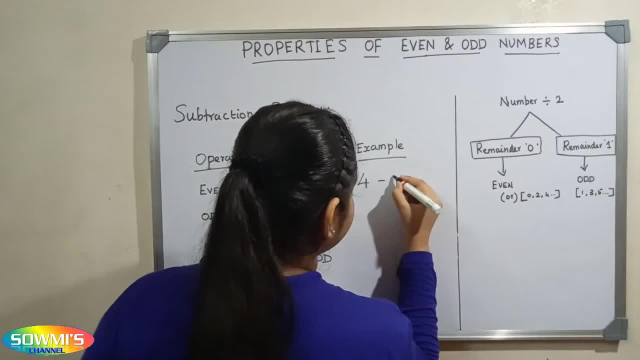 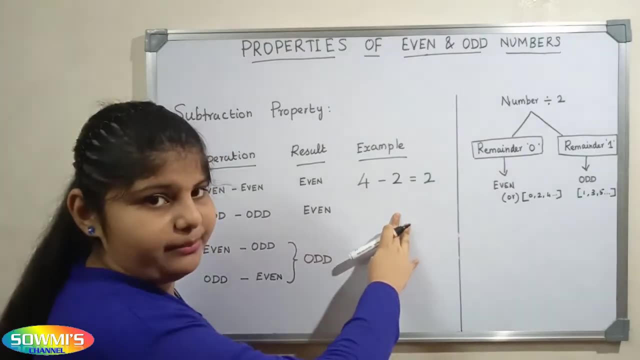 For example, we can take: 4 minus 2 is equal to 2.. Here 4 and 2 are the two even numbers. When we subtract 4 from 2, we will get the result as 2.. 2 is an even number. 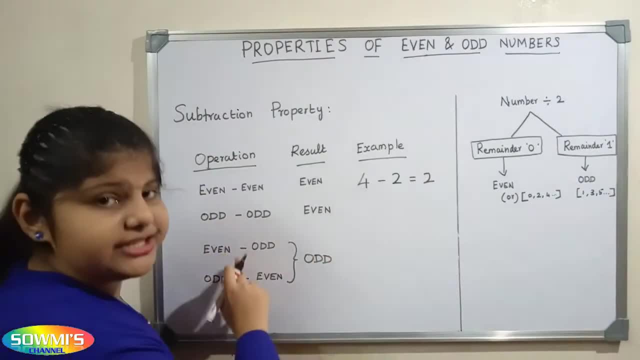 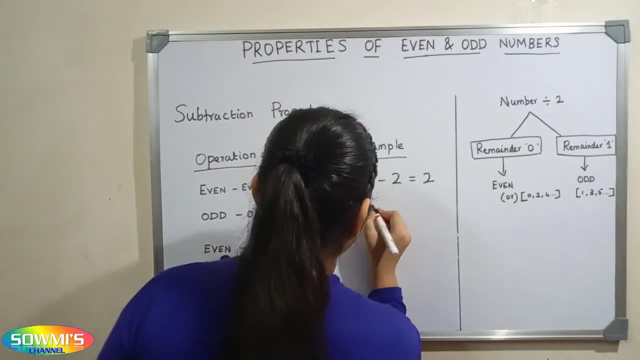 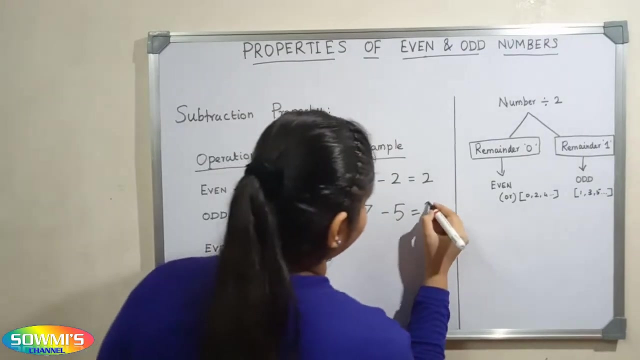 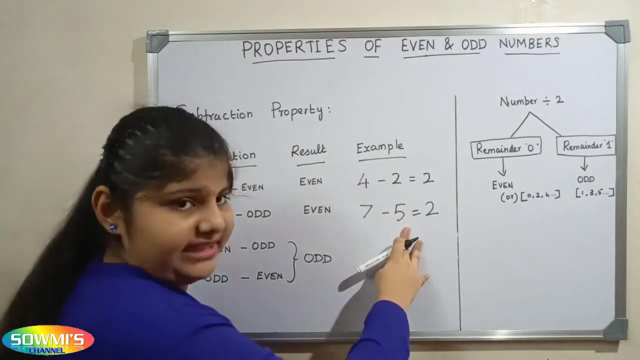 Subtraction property. When we subtract two odd numbers, we will get the result as an even number. For example, we can take: 7 minus 5 is equal to 2.. Here, 7 and 5 are the two odd numbers. When we subtract 7 from 5, we will get the result as 2.. 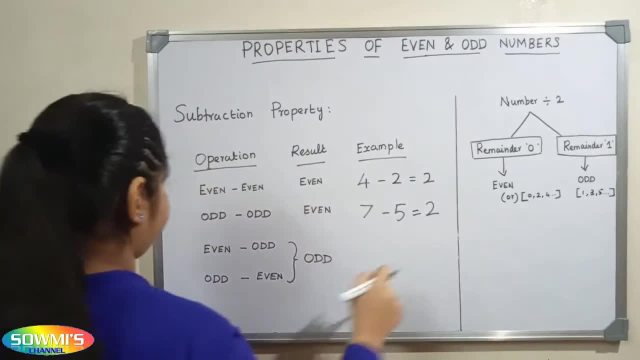 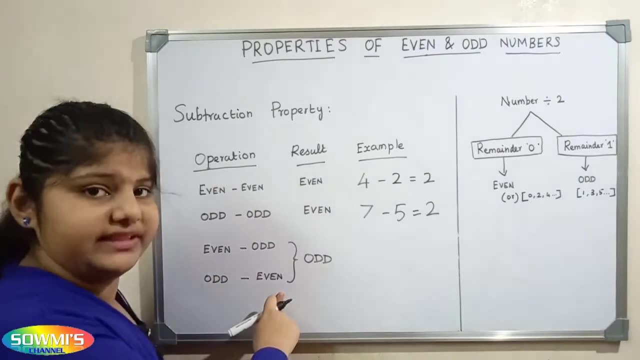 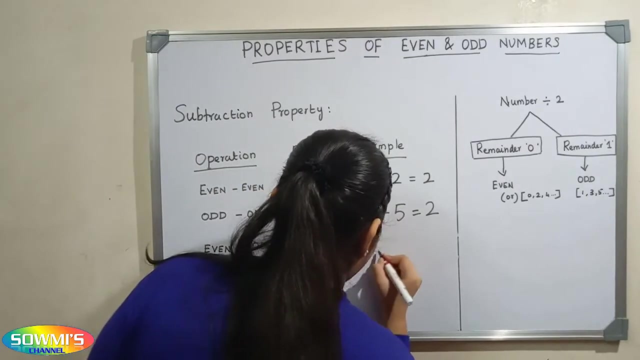 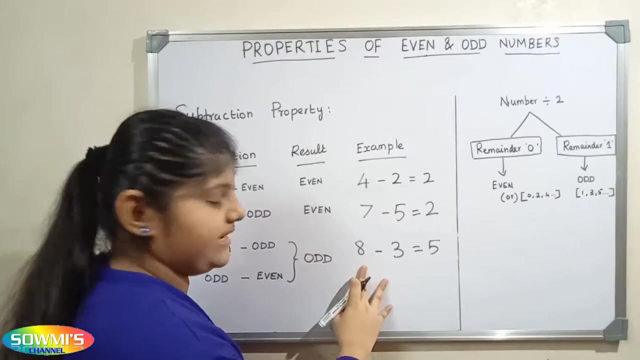 Here 2 is the even number. When we subtract even number from the odd number or odd number from the even number, we will get the result as an odd number. For example, we can take: 8 minus 3 is equal to 5.. Here 8 is an even number and 3 is an odd number. 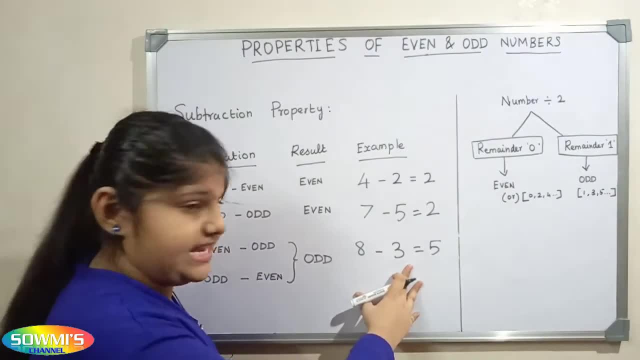 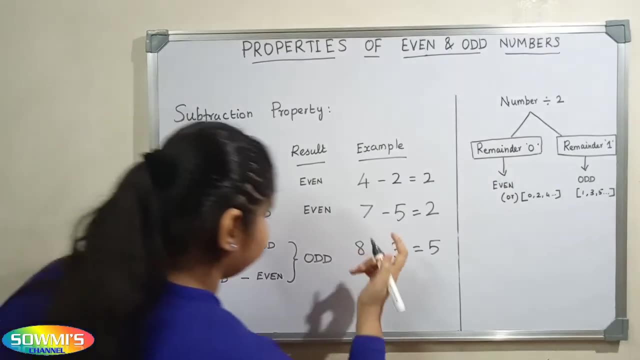 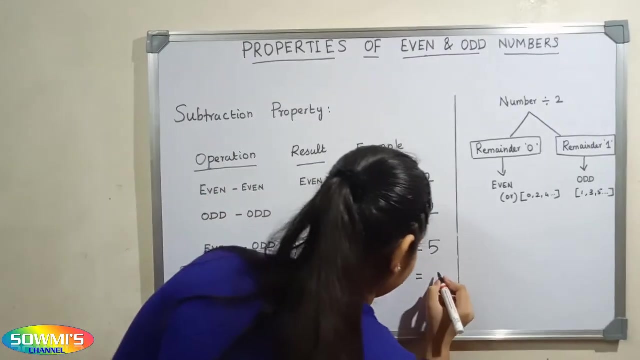 When we subtract 8 from 3, we will get the result as 5.. Here 5 is the odd number. Next we will take one more example: 9 minus 2 is equal to 7.. Here 9 is the odd number and 2 is the even number. 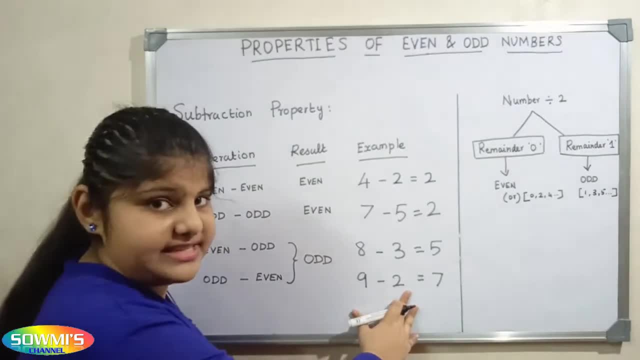 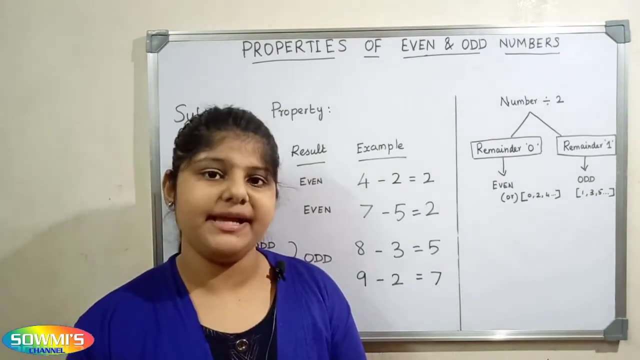 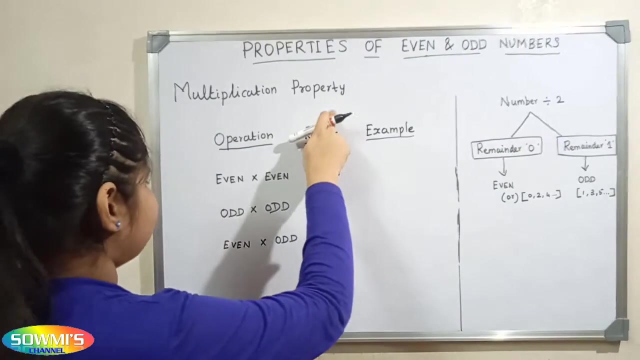 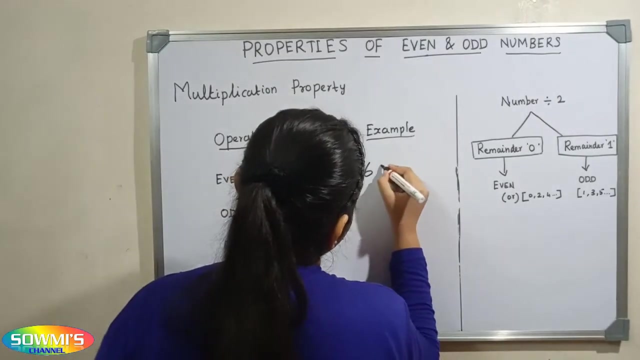 When we subtract 9 from 2, we will get the result as 7.. Here 7 is the odd number. Next we will see multiplication property. When we multiply two even numbers, the result will be an even number. For example, we can take 6 multiplied 4 is equal to 24..